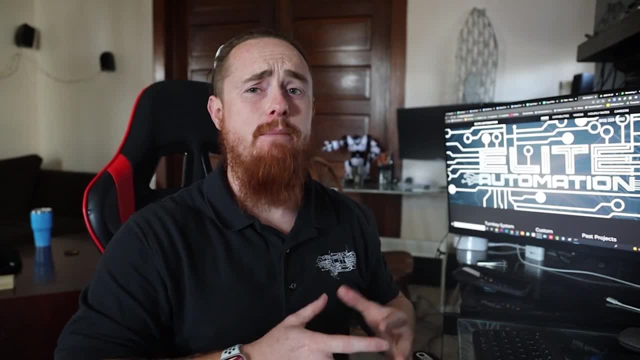 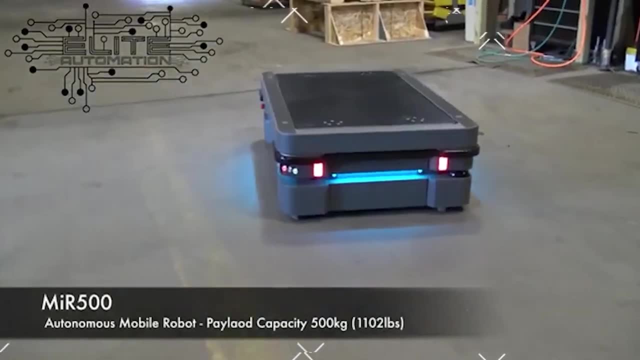 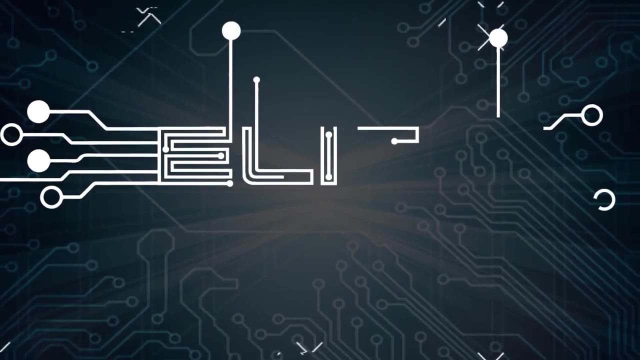 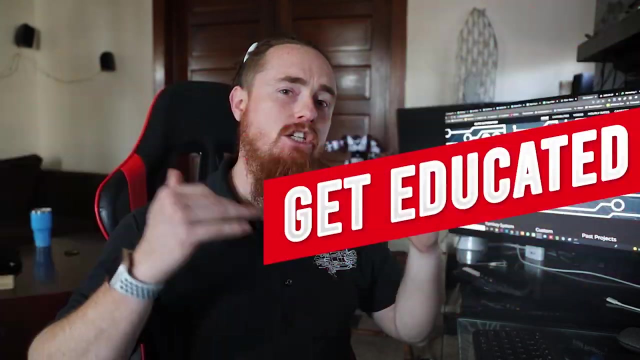 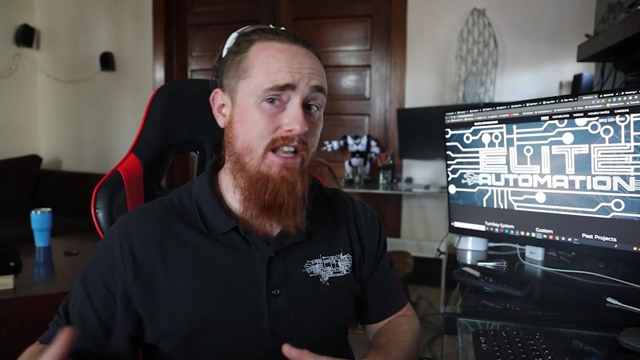 Hi, how's it going? I'm Malachi Greb, CEO and engineer of Elite Automation. Today, I want to talk to you guys about the best way to get educated in automation, And this will be specifically for somebody who may be still in high school or is just now getting. 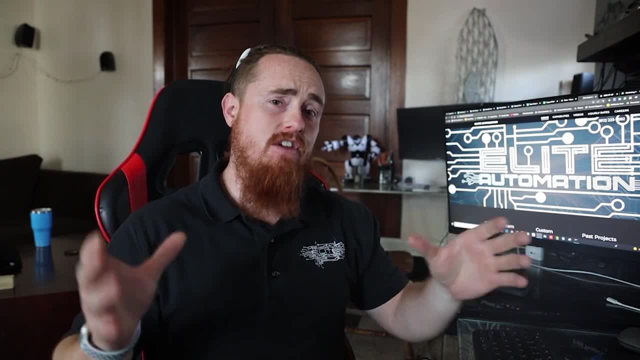 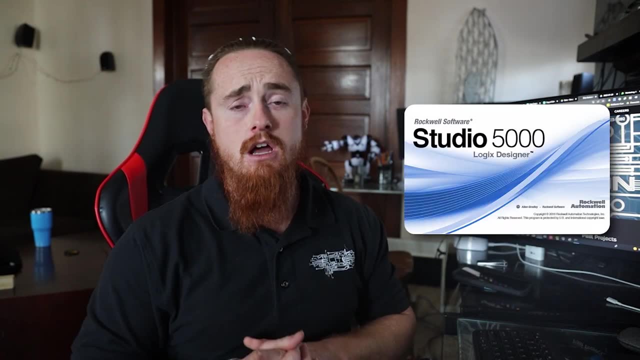 into college And that is target on a specific piece of software. So if you're doing PLC, I would suggest you do Studio 5000, Alan Bradley's software, which is going to be expensive. It's going to be hard to get your hands on it. You can do a trial but that's only going to give you. 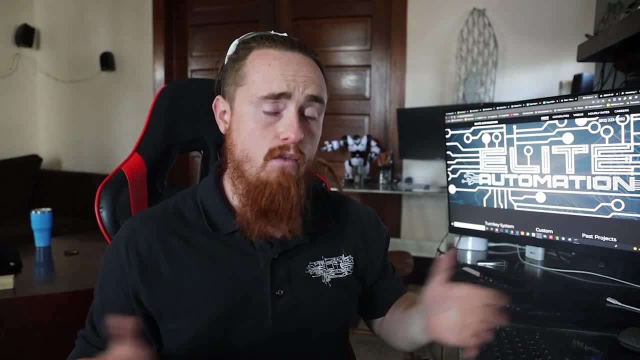 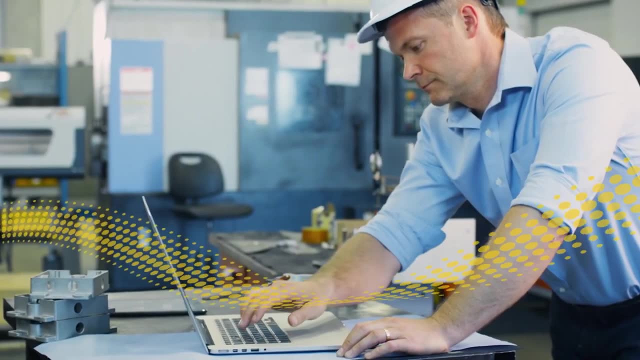 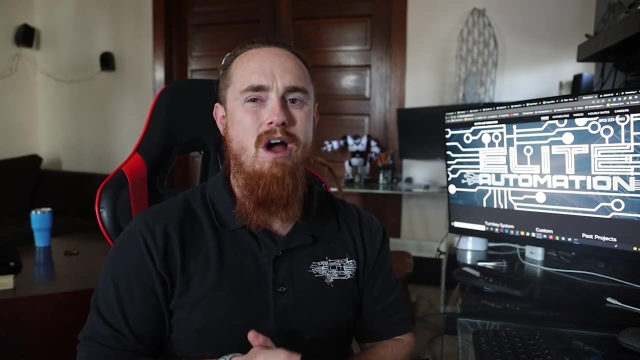 like seven days. There are other free PLC softwares out there, but Alan Bradley's the number one brand here in the United States. If you're outside of the United States, I would suggest Siemens And just look into the most popular PLC brands and that will tell you what PLCs to practice with. 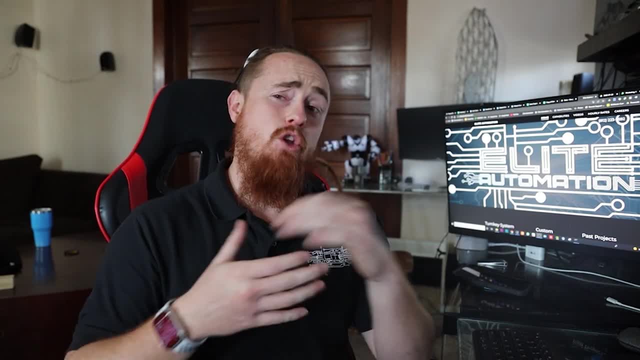 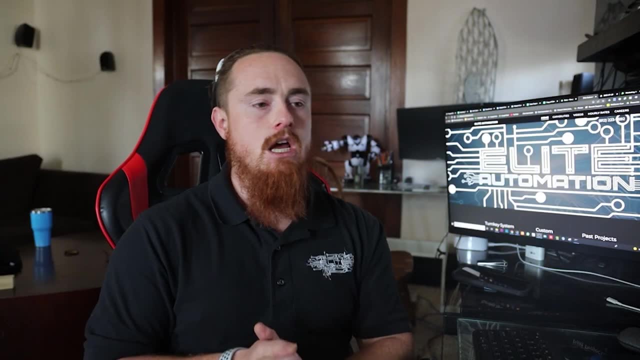 Then the next thing you can do is robot programming. So if you're in the United States, I would highly suggest that you use FANUC robots. They're the number one robot here in the United States. You can download a software called RoboGuide. I believe they'll give it to you. 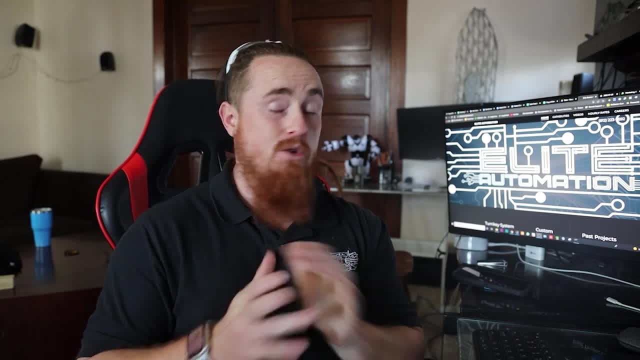 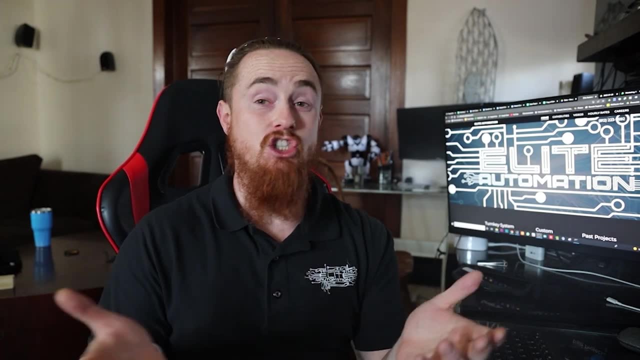 and let you try it out on a 30-day basis. So if you're in the United States I would suggest a 30-day trial. Don't tell FANUC I said this, but you can buy another computer and download that 30-day trial again, So you can have like a bunch of just cheap computers And it's a lot cheaper. 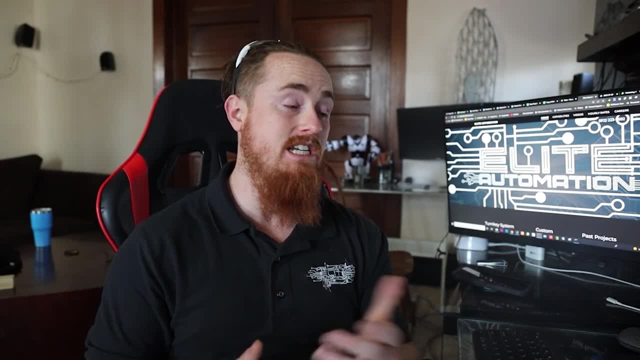 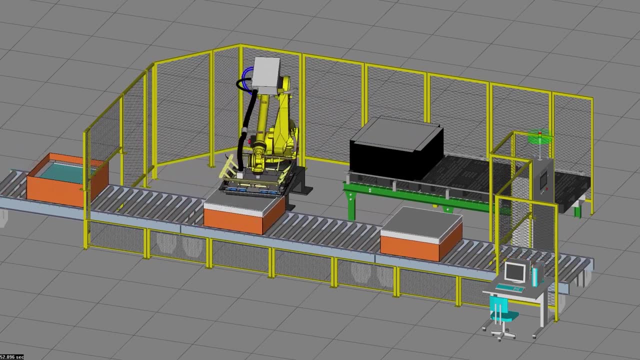 than the software, because the software, I think, is like $2,000 a year per seat. Unless you're willing to make that type of investment, it's definitely worth it. I would rather you buy a $2,000 seat of FANUC, RoboGuide or Alan Bradley software- any of these expensive softwares. 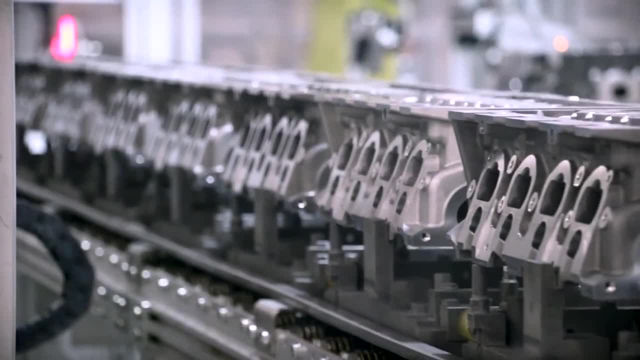 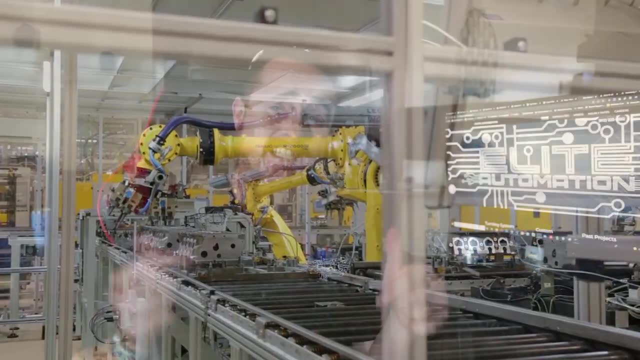 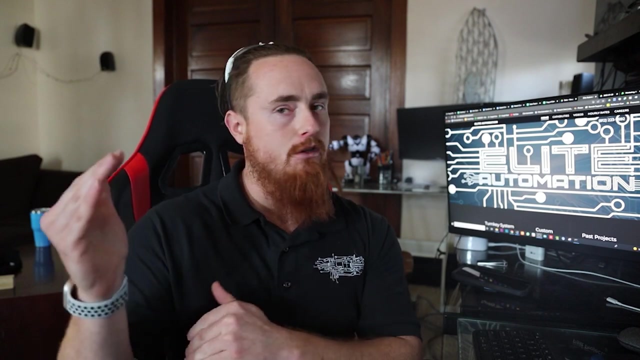 I'd rather you do that than honestly take a college course And then just watch tutorials. subscribe to YouTube channels like this one that'll teach you how to use some of those softwares. Ask comments down in the comments below so we can make more videos like that to help you guys out. But outside of that, look up most popular robot. 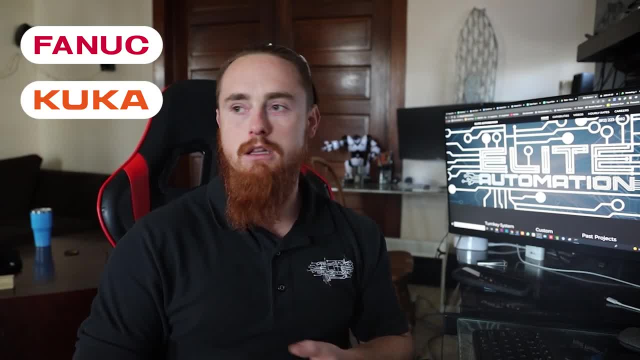 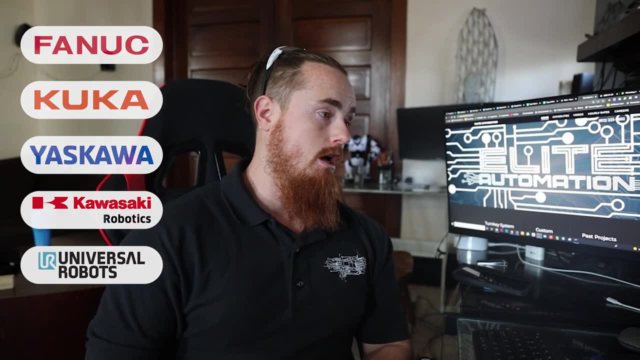 brands: FANUC, KUKA- let's see Yaskawa, Kawasaki, UR Robots are becoming really popular Collaborative robot, So just take a look in that And some of these other you might be able to find. 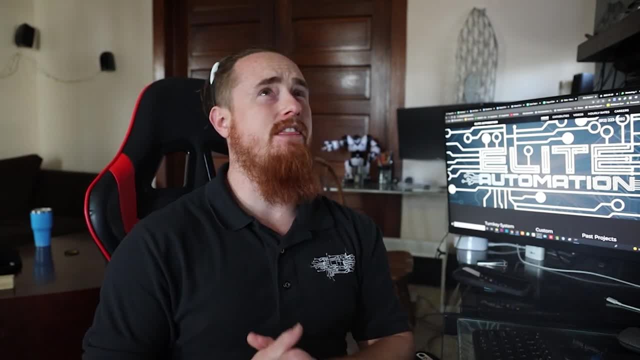 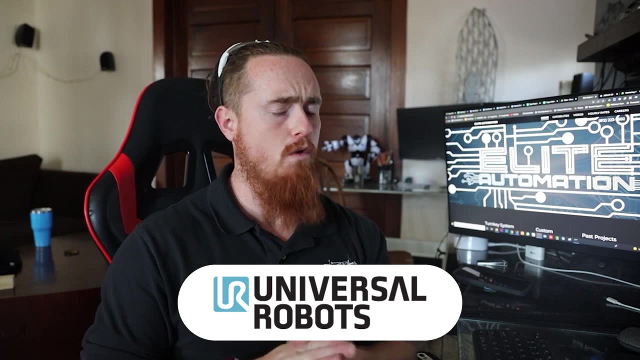 other robot programming software that's actually free. I think you can actually get UR Robots for free. I've definitely used a simulated version of UR Robot, So you might be able to get that one, which would be a really good one to learn, since it's popularity in the market. Then, whenever it, 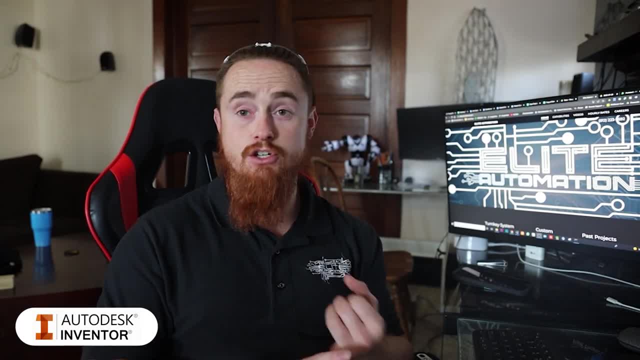 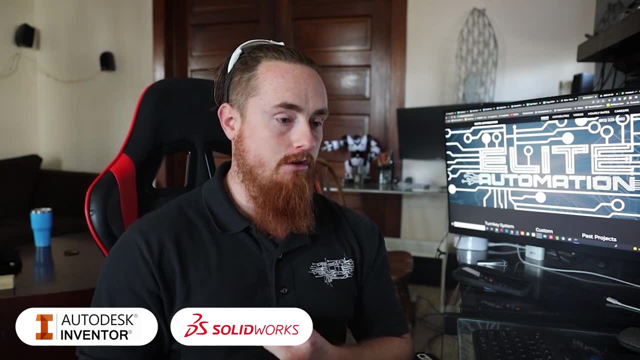 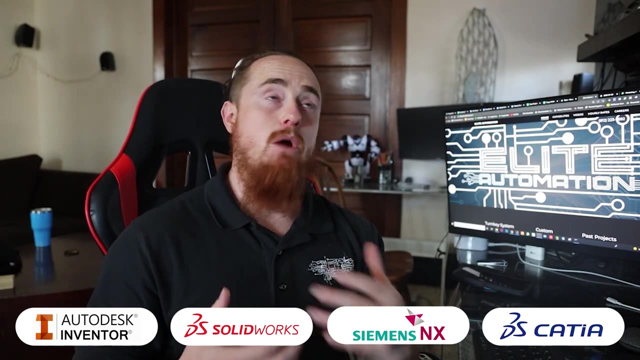 comes to mechanical engineering, I would definitely be focusing on Inventor. I'd be focusing on SolidWorks. Both of them are very, very popular in the industry. There's definitely some other softwares. I'm trying to think. I'm not a mechanical engineer myself, but I work at TIA, But I work with a lot of. 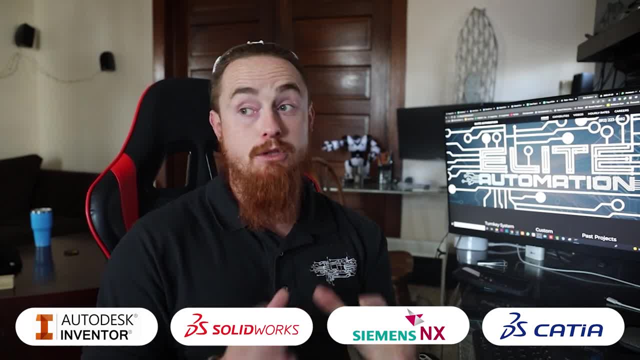 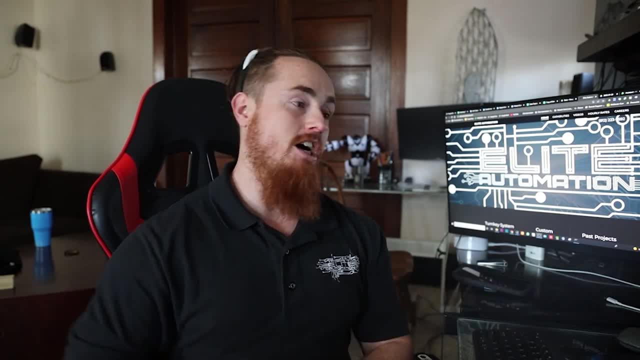 engineers and working with different softwares and things like that. But some of those softwares are extremely expensive And unless you're looking to get a cracked version and do some illegal stuff, which I don't, suggest those softwares- some of them, are extremely expensive. But Inventor and 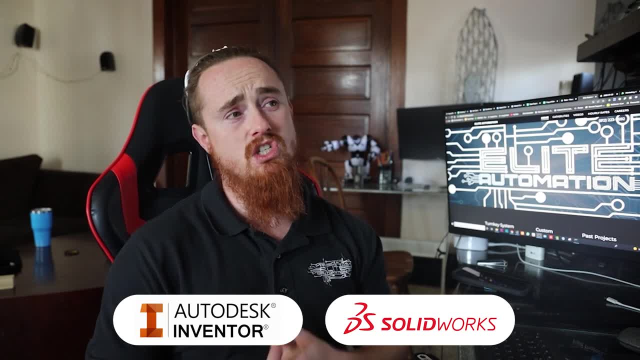 SolidWorks are fairly doable. You can do like a subscription service And also, if you go to college, you can do like an education package, And some of them even offer it for free if you're going to college, So it might be worth. 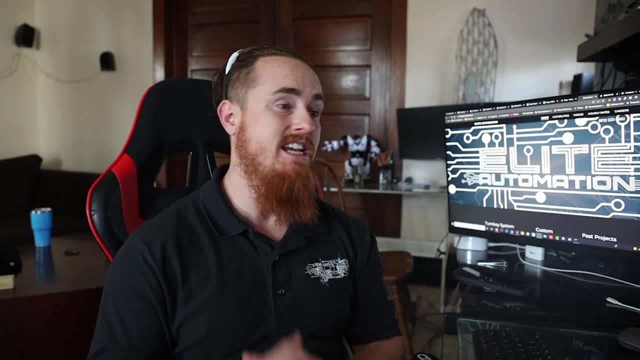 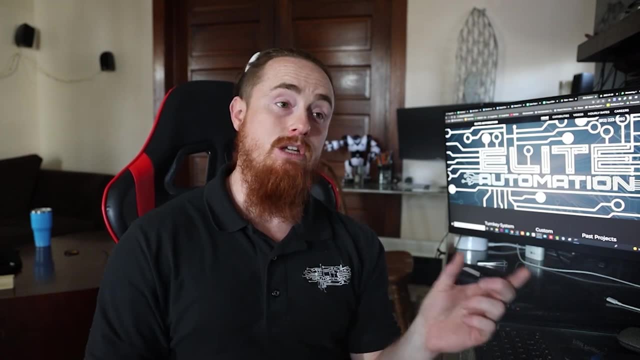 signing up for, like, a college course, getting a college email ID and then getting that free software to go along with it. Even if you only take one course, I think you can get a like a college email ID which would give you a free access to those softwares for a couple of years. 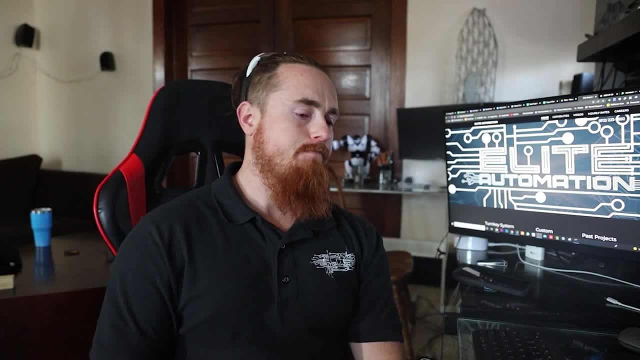 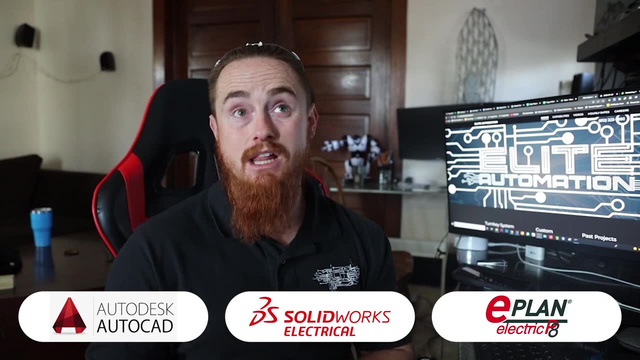 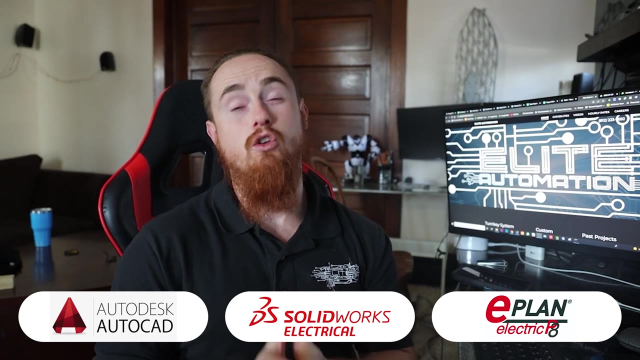 And maybe some of the other softwares will start doing that over time as well. Let's see Electrical engineering would be maybe AutoCAD, Electrical SolidWorks, Electrical Eplan. Those are all three softwares that are very, very popular. There's definitely some more out there. I'm just not all too familiar with the different softwares. 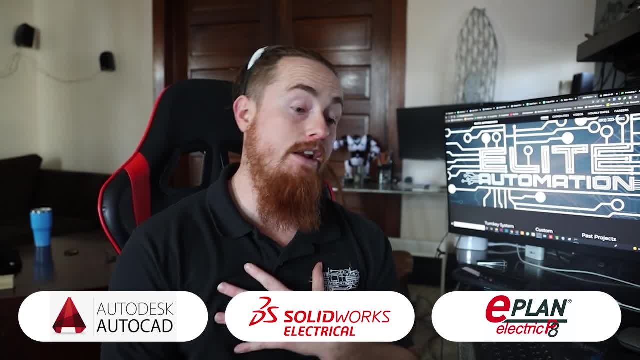 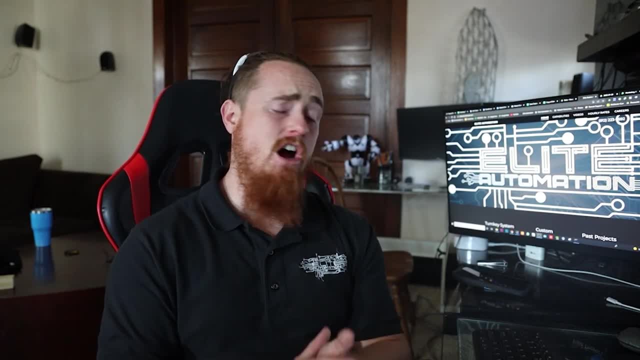 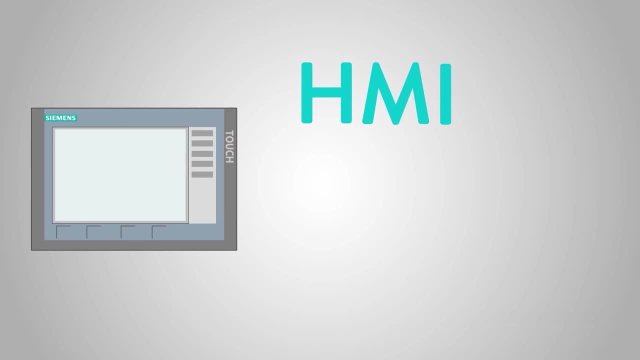 on the market for electrical engineering. Even though I have done electrical engineering, I've primarily done it in the AutoCAD Electrical Realistically guys. I think that kind of covers at least the mechanical, electrical and software side of things. Also, HMIs is another good one to program and develop on. You want to do like some?